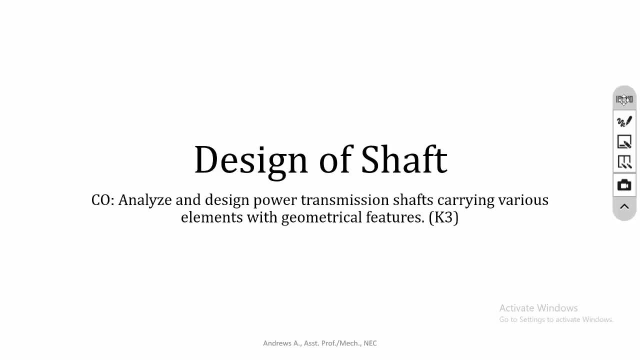 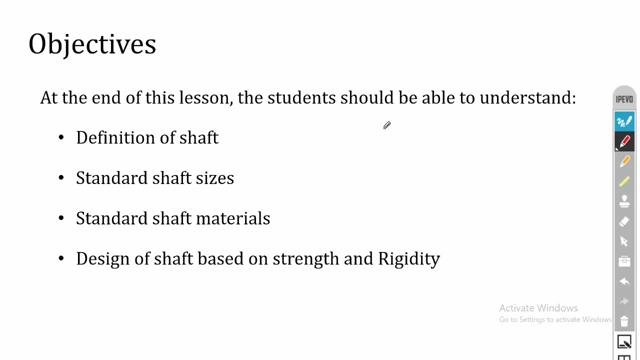 In this lecture I am going to start the second CO: Design of Shaft. The CO statement is Analyze and design power transmission shafts carrying various elements with geometrical features, And the CO level is K3 level. So the objective of this lesson is: at the end of this lesson the students will be able to understand definition of shaft, then standard shaft sizes, then standard shaft materials. finally, design of shaft based on strength and based on rigidity. 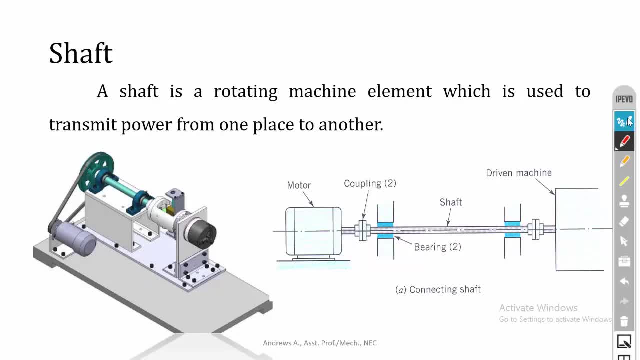 So, first of all, what is in the shaft? So a shaft is a rotating element That is used to transmit the power from one machine component to other one. So, generally, the shafts are used to transmit power between the motor and a machine. 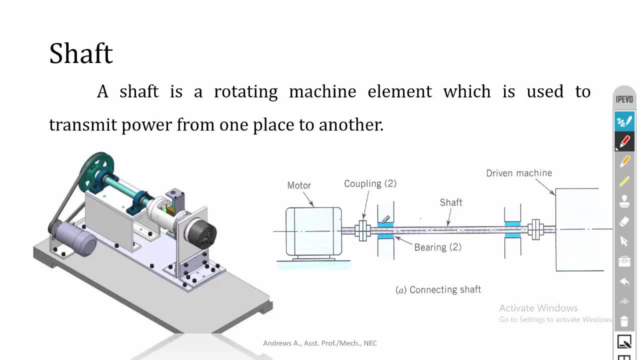 Maybe in a centrifugal pump. the shaft is used to transmit the power between the motor and the centrifugal pump. So that is how the shaft is transmitting the power, and the shaft is supported in bearings. So because of transmission of the power, the shaft is subjected to twisting moment, that is, torque. 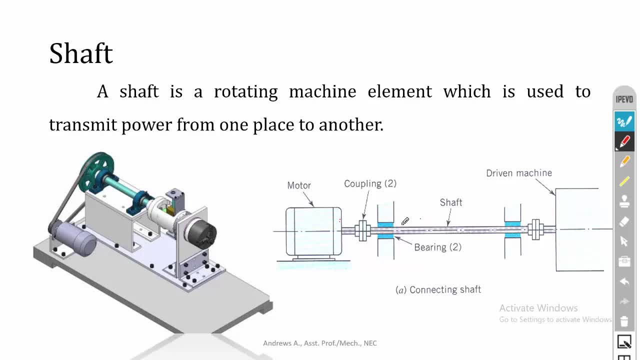 And the shaft carries some pulleys and some gears, So those pulleys and gears are subjected to transverse load. So the shaft is also subjected to transverse load. So when you are designing a shaft, we have to keep all the loads into consideration and finally, we have to calculate the diameter of the shaft. 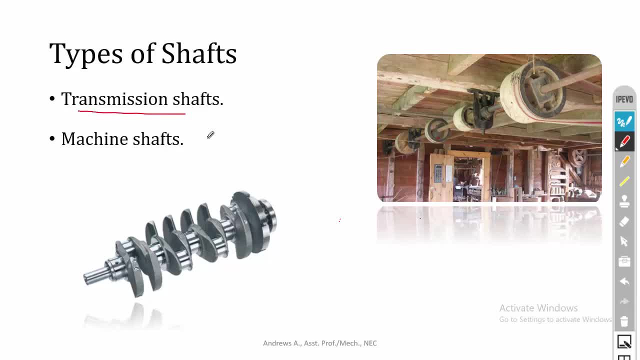 There are two types of shafts are there. The first one is a transmission shaft and the second one is a machine shaft. So the transmission shaft is used to transmit power between various elements. So in your floor mill you can see that a single shaft is used to transmit the power between. 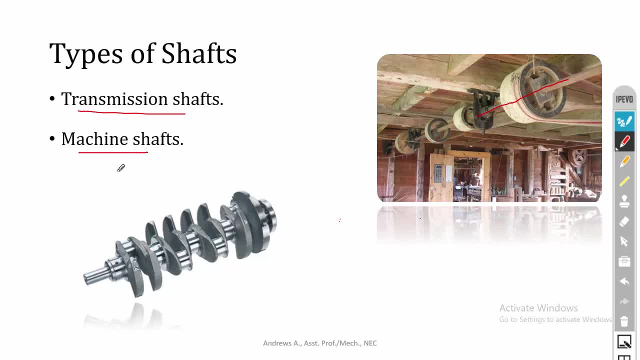 A motor and various floor mills And in machine shaft. so this is the integrated component of a machine. The example for a machine shaft is a crank shaft or a cam shaft, So these shafts are integrated to do some useful work inside a machine. 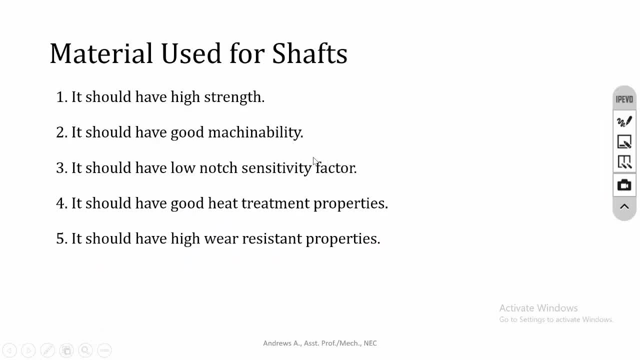 So that is why it is called as machine shafts. So the material used for shaft should have high strength. It should have have good machinability because we are going to fix the pulleys and gears in the shaft. then it should have low notch sensitivity factor. ok, to fix the pulleys and gears we. 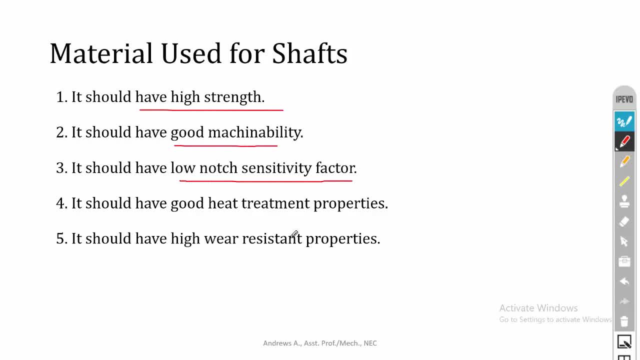 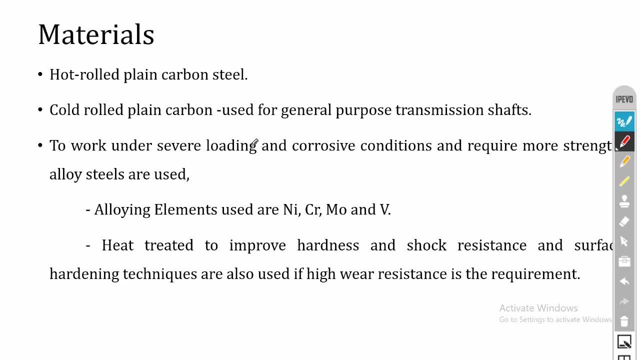 are going to groove the keyways, ok, so the shaft should have a low notch sensitivity factor. then it should have a good heat treatment properties. finally, it should have high wear resistance properties. so there are some standard materials are used for shaft. the first one, hot rolled plain carbon. 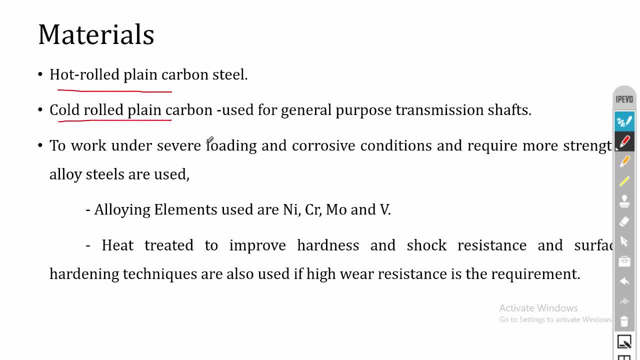 steel and further the cold rolled plain carbon steel can be used for general purpose transmission shaft. Then, in case of the shaft is working under severe loading and corrosive environments, then we can go for alloy steel elements. so generally the alloy steels which are used for shafts, it is generally had a very listening finish weight for now should be almost, almost. 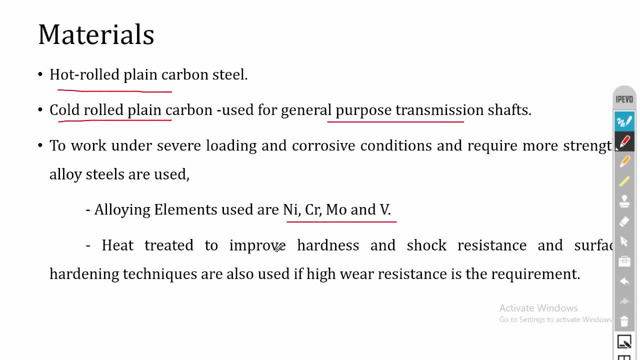 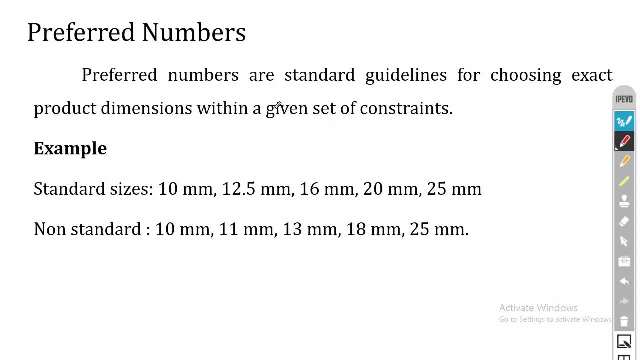 shaft manufacture is nickel, chromium, molybdenum and vanadium. Preferred numbers are some standard guidelines for shaft diameters. So the preferred numbers have some standard set of numbers. So we have to select the diameters according to these standard numbers. 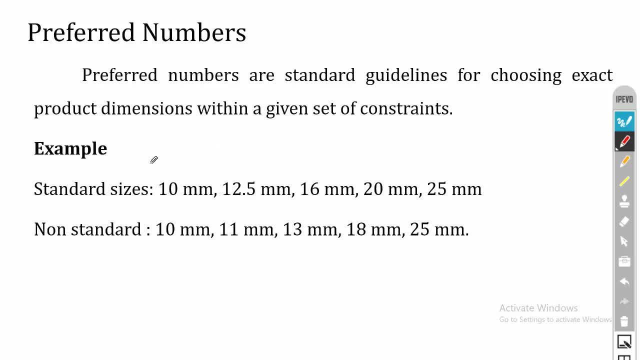 For example, I am going to fix a standard in between 10 mm to 25 mm. So if you take the standard sizes, then it is 10 mm, then it is 12.5 mm, then 16 mm, 20 mm and 25 mm. 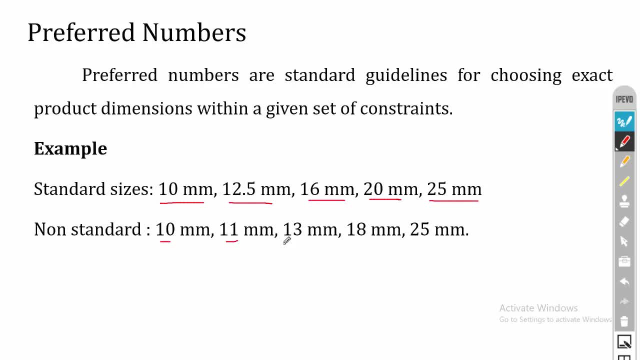 In case of non-standard, it is 10,, 11,, may be 12,, 13,, 17,, 18,, whatever it may be. So, for example, I am going to select a shaft with a diameter of 11 mm. 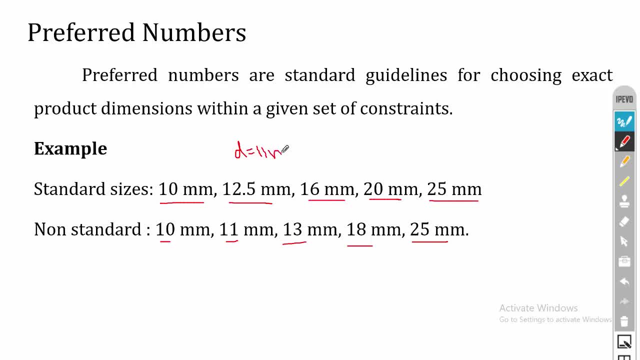 The final answer in the problem is: D is equal to 11 mm. Okay, So when you are going for standardization, then you have to go for the next higher standard diameter. So if the D is 11, then you have to select the diameter of 12.5 mm. 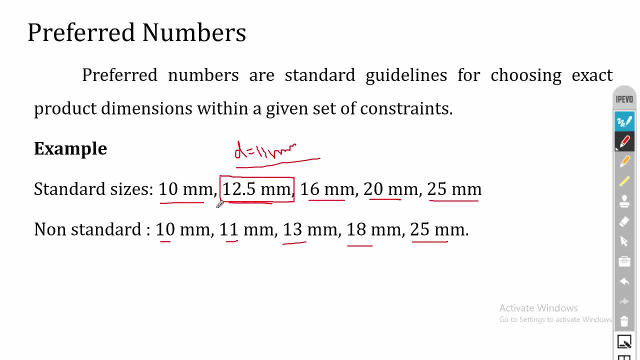 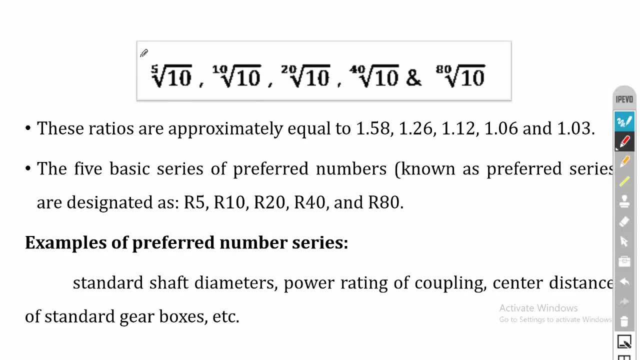 So this is how you have to use the preferred numbers while selecting the shaft diameter. So there are five preferred numbers, are there? So these are all the five. So the ratios are approximately equal to 1.58 for the first one, And for the second one it is 1.28.. 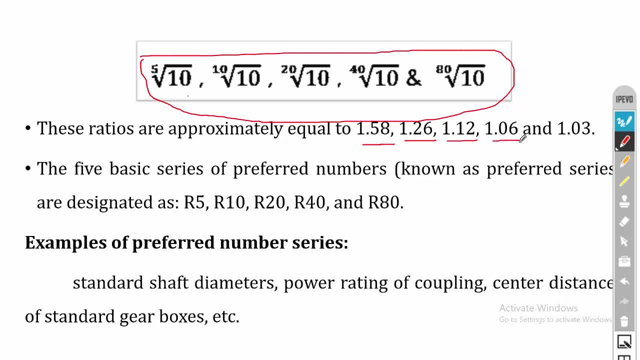 And for the third one it is 1.12.. Then for the fourth one it is 1.06 and for the last one it is 1.03.. So these five preferred numbers are further named as R5, R10, R20, R40 and R80. 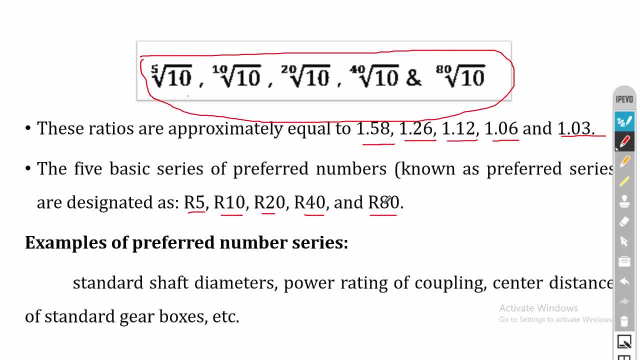 So these five numbers are used in machine design to select the standard component sizes. Okay, Okay. So these are all some of the examples for standard preferred numbers. The first one is shaft diameters. So the preferred numbers can be used for selecting the standard shaft diameters. 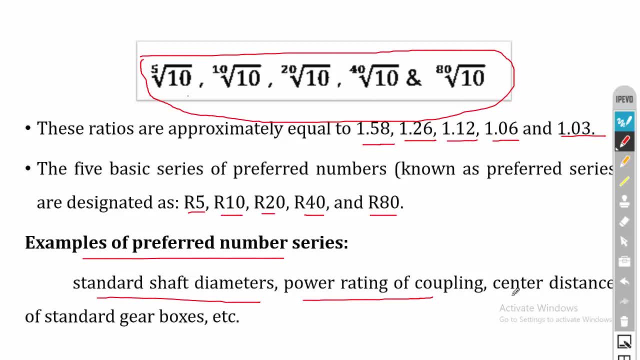 Then the power rating for a coupling Further for center distance of standard gear boxes. Okay, While calculating, while selecting this center distance for any gear box, then we can use these preferred numbers for selecting the standard center distance value. Okay, So in this CO we are going to use the preferred number for standard shaft diameters. 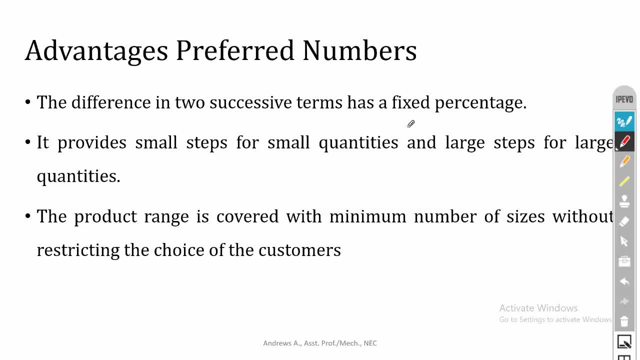 Then the advantages of preferred numbers is so there is a fixed percentage between two successive terms. Then, for small quantities, it provides small steps and large steps for large quantities. So in between 1 and 10. Okay, It has some small step values, and in between 10 to 100, it has some large step values. 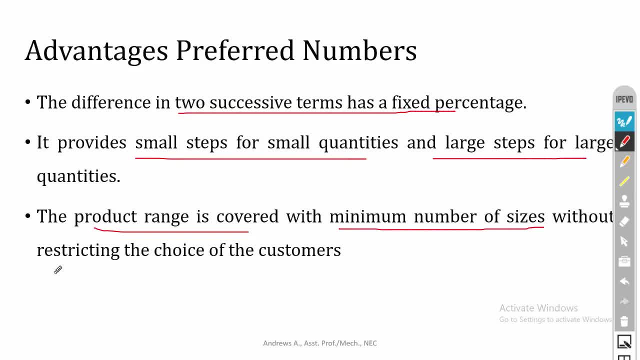 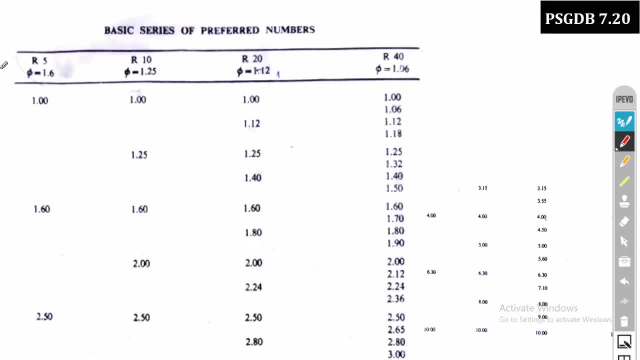 Then the product range is covered with minimum number of sizes, without resting the choice of the customers. So these are all the preferred series given in your data book. So it is in the page number 7.20.. So R5, R10, R20 and R40 is given in the data book. 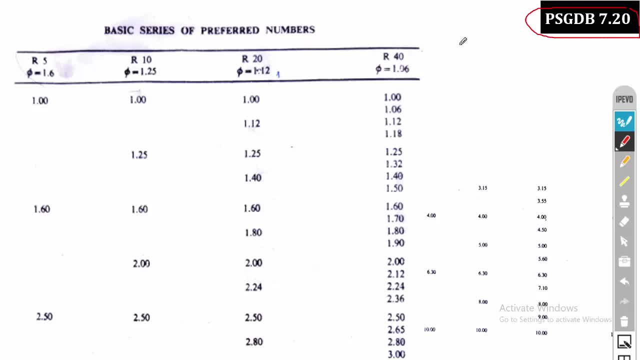 Okay, And for shaft diameters. so generally we will use R20 series. So these are all the preferred sizes. Then, from 2.8, then it is 3.15,, 4,, 5,, 6.3.. 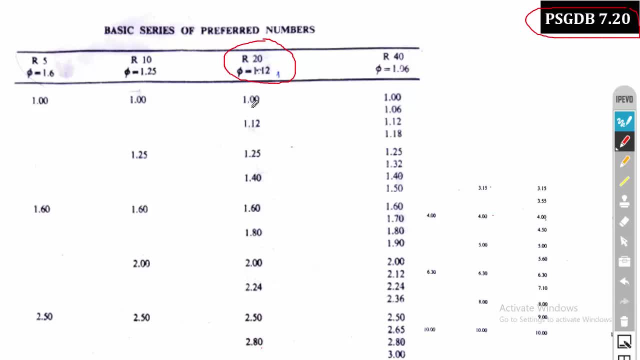 Then it continues. Okay, So for the first cycle it is from 1 to 10.. And in the case of second cycle, then you can multiply 10 with this. Okay, Then for the second cycle it starts from 10,, 11.2,, 12.5,, 10.5,, 10.5,, 10.5,, 10.5,, 10.5,. 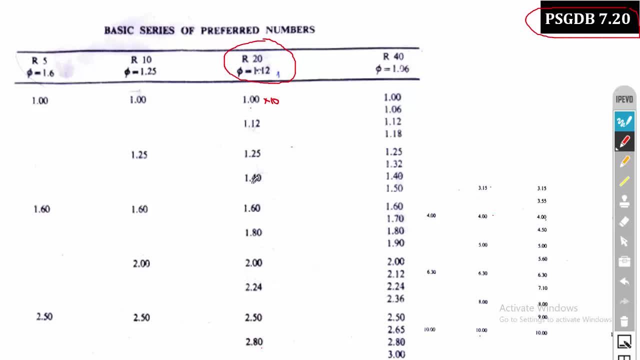 10.5,, 11.2,, 12.5,, 14,, 16,, 18, and it goes on. So let us assume a calculated diameter of 21 mm. Okay, So the final answer is D is equal to 21.. 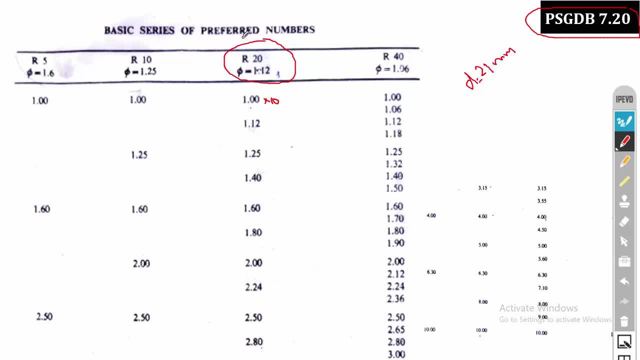 Okay, So what I am going to do is I am going to use the R20 series for selecting the standard diameter. Okay, So let us look into the R20 series. The first series is from 1 to 10.. In the second one, you just multiply 10 with this. 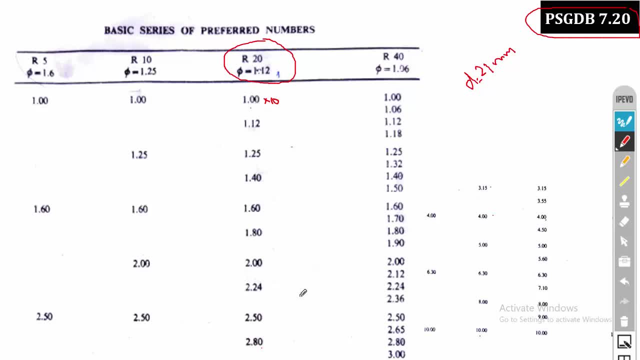 So you will get 10,, 11.2, like that. Okay, So our diameter value is 21 mm. So you can see here. So here it is 20 and here it is 22.4.. Since our diameter is 21 mm, then we have to select the next standard diameter. 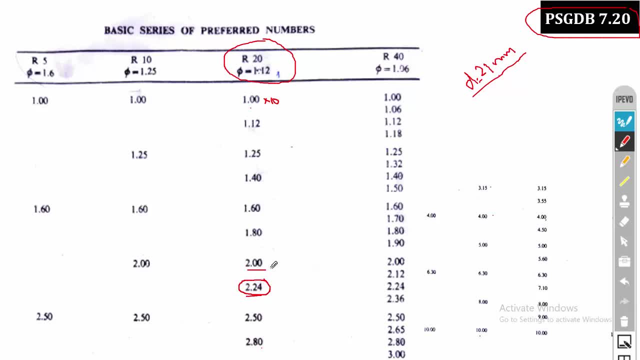 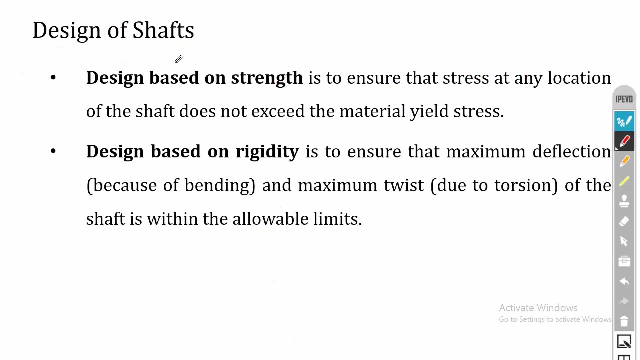 Okay, So the standard diameter is equal to 10.5.. Okay, So our diameter is equal to 22.4.. So standard D is equal to 22.4 mm. So this is how we have to use the preferred numbers in selection of the standard diameters. 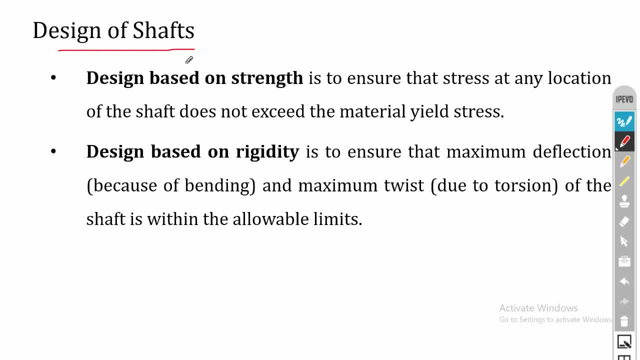 Then coming to the design of shafts. So the shafts are designed based on two things: one is strength and the second one is rigidity. So in the case of strength, the shaft is designed by considering the yield strength. So at any location, the shaft should not exceed the yield strength of the material. 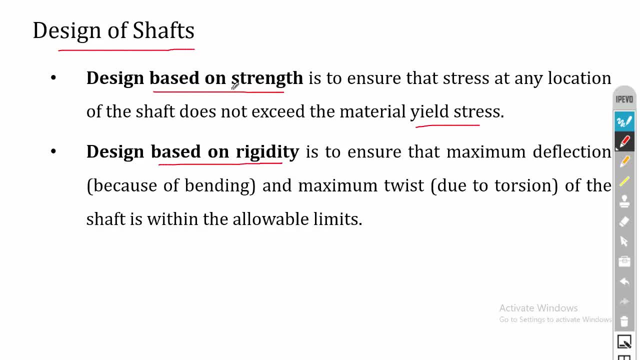 So if it exceeds the yield strength of the material, then the shaft will fail. So that is the design based on strength. Then the second one is the design based on rigidity. So in this case we have to design the shaft based on the maximum deflection and the maximum. 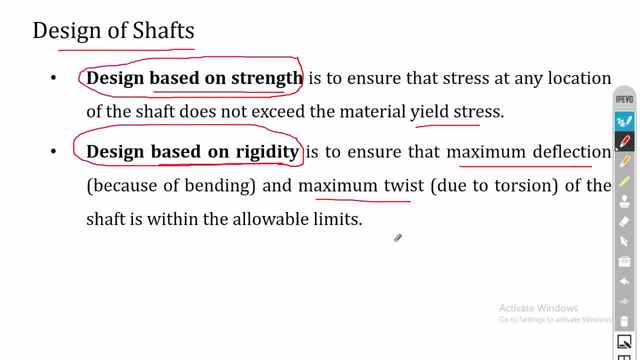 twisting. So deflection in the case of bending and twisting in the case of torsion. Because in some of the shafts, some gears are placed in the shaft to transmit the power. So if the shaft exceeds some standard bending, Then what will happen is there will be a improper meshing between the two mating gears. 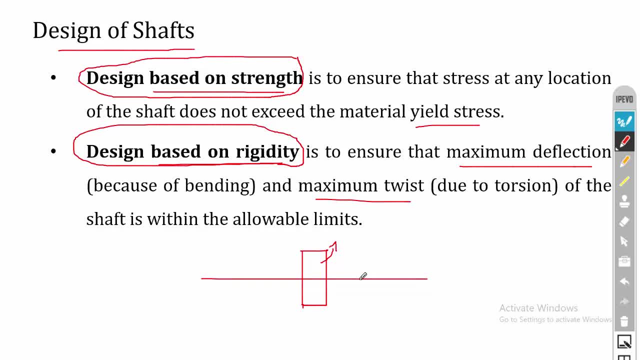 So the gears will produce some high amount of noise and vibration, So that will damage the system. So you have to consider the deflection also into consideration And in some cases the shafts are designed based on both strength as well as rigidity. 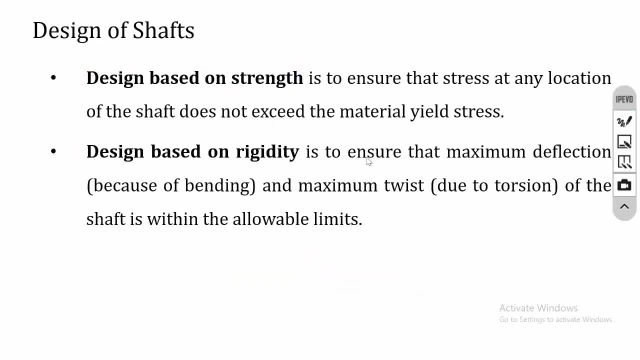 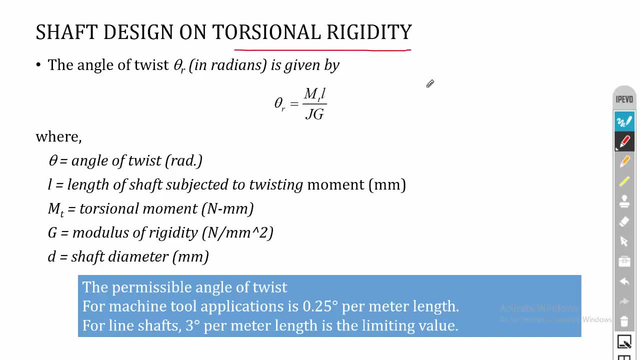 So this is how we have to design the shaft. So in the case of shaft design based on rigidity, then we know that the torsion equation is: t by j is equal to gdeta by l, So in the case of t, we can use mt hereafter. that is the torque. 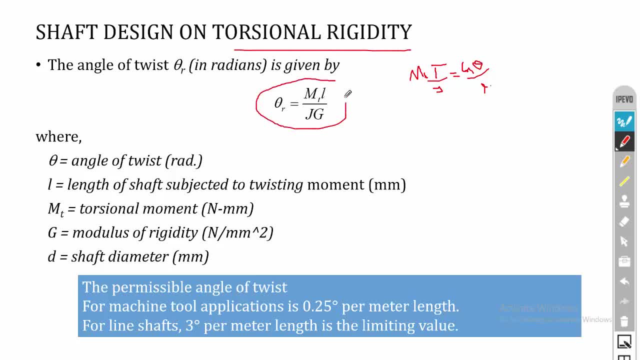 So if you keep the theta in the left side Then you will get this equation: d theta is equal to mt l divided by j into g. So here m is the, t is the twisting moment in Newton. mm. L is the length of the shaft. 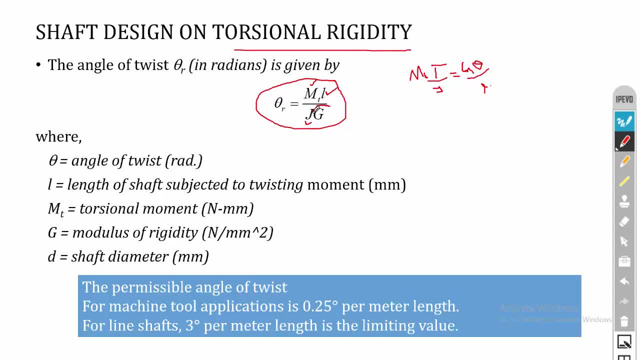 Then j is the polar moment of inertia And g is the modulus of rigidity in Newton per mm square. So if you substitute everything, finally you will get d theta in radian. Okay, So there are some. Okay, some permissible data values are there. so here you can see that for machine tool application. 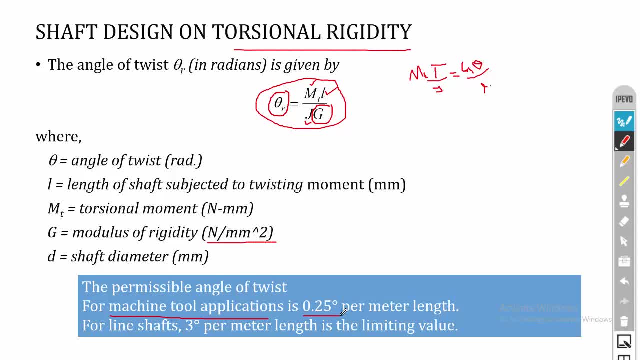 the permissible data value is 0.25 degree per meter length, so this is the maximum limit. and in the case of line shaft, the angle of twist limit is 3dta per meter length. so these are all the permissible angle of twist values, so you can use this equation to design a shaft. 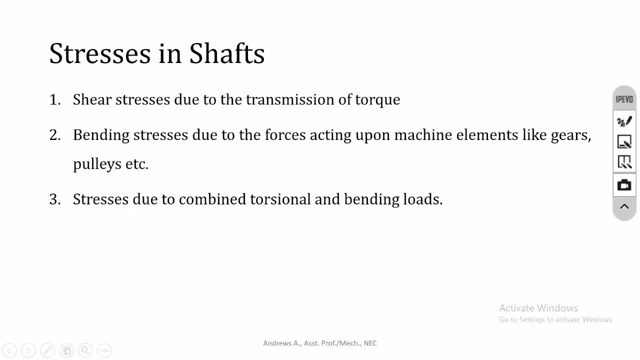 based on the rigidity. The next one is design of shaft based on strength. in strength basis, there are three type of stresses are acting in the shaft. the first one is shear stress due to transmission of torque. so the main purpose of the shaft is to transmit the power. 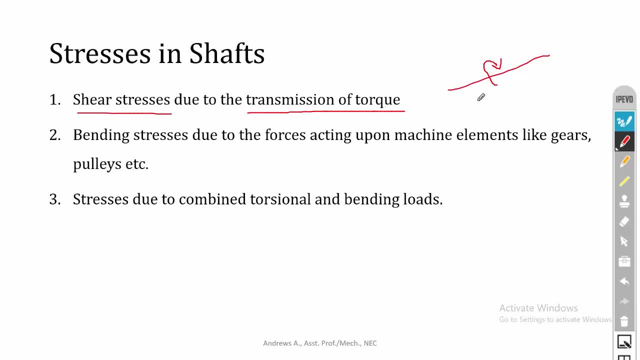 So while transmitting the power, the shaft is subjected to some twisting moment or torque. so the shear stress is induced when the shaft is subjected to torque. so this is the first stress. Then the second stress is bending stress due to the forces acting upon machine elements. 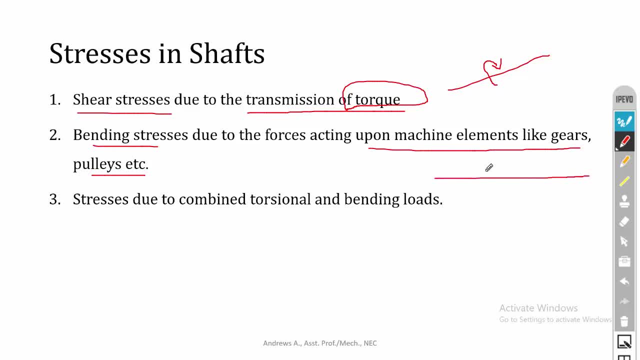 like gears and pulleys. so the shaft carries pulleys and gears in its span. so when the pulleys and gears are placed in the shaft, then these pulleys and gears are subjected to some external forces, so these forces will create a bending stress on the shaft. so because 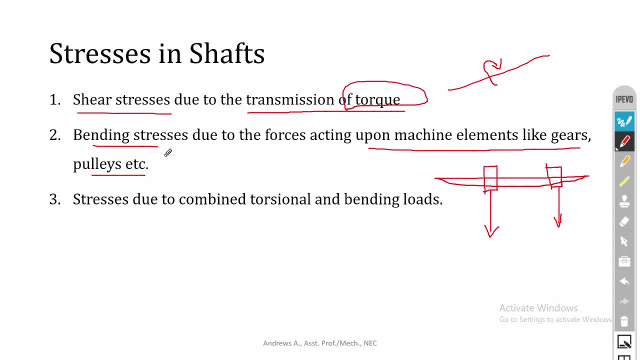 of the pulley and gear, the shaft is subjected to bending stress. so that is the second one, And the third one is stresses due to combined torsional and bending. so in this case the shaft transmits power And also the shaft carries some pulleys in its span. so here, because of the pulley, the 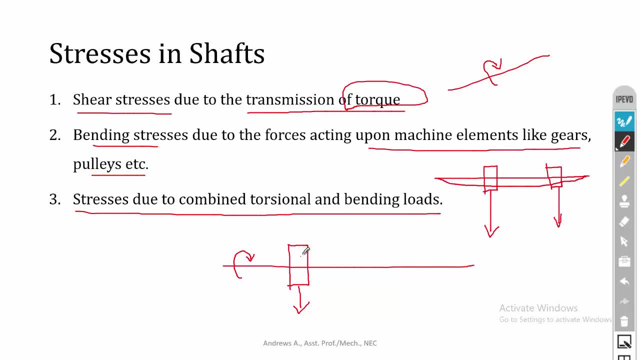 shaft is subjected to. maybe because of the pulley or gear, the shaft is subjected to bending and because of the twisting moment the shaft is subjected to shear stress. so that is combined bending and shear stress. and this is the important one, because in most of the cases the shaft 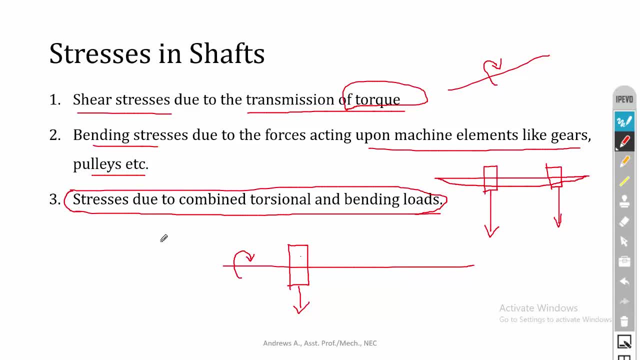 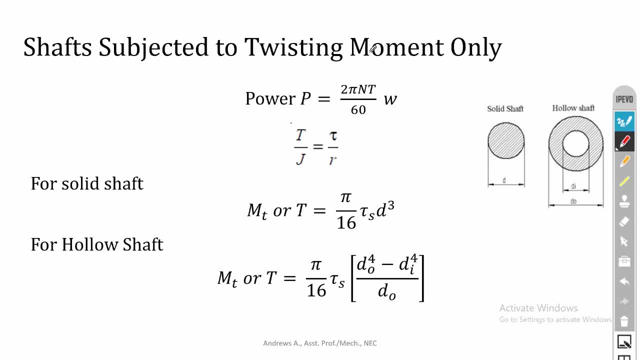 is subjected to both bending and twisting. So we will start from shaft, subjected to twisting moment only. we know that the equation for power is P equal to 2 pi nT divided by 60, so P is power in watt and n is speed in. 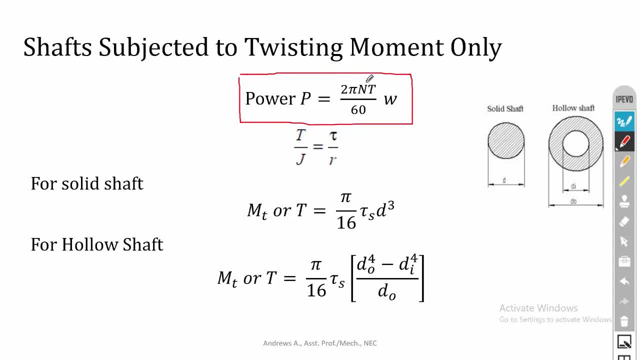 rpm. T is torque in Newton meter. then further for solid shaft. we already know that mT is pi by 16 tau into d cube. so you can substitute the j value and r value in the shear equation. finally you will get the mt value. so mt is equal to pi by 16 tau into d cube in the case of solid. 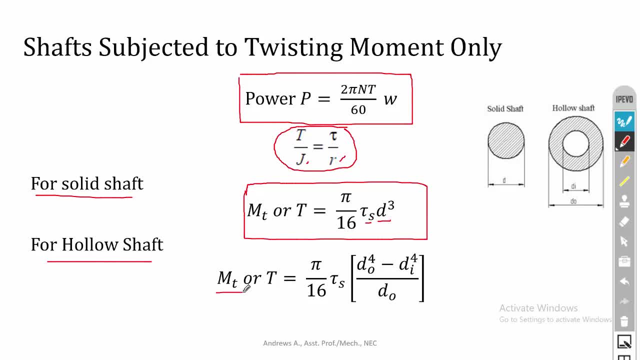 shaft and in the case of hollow shaft, then mt is equal to pi by 16 tau. outer diameter: power 4 minus inner diameter. power 4 divided by do, you can see that do is outer diameter and di is inner diameter. okay, so this is for shaft subjected to twisting moment only, and we have solved some. 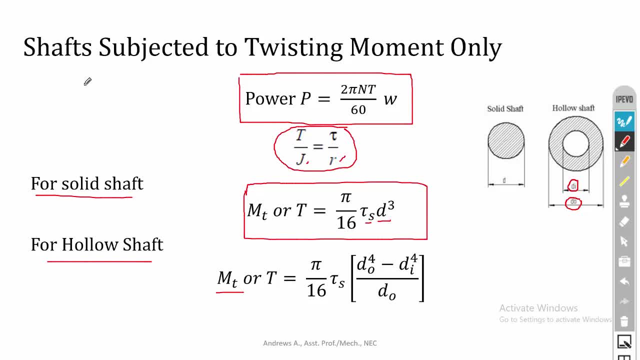 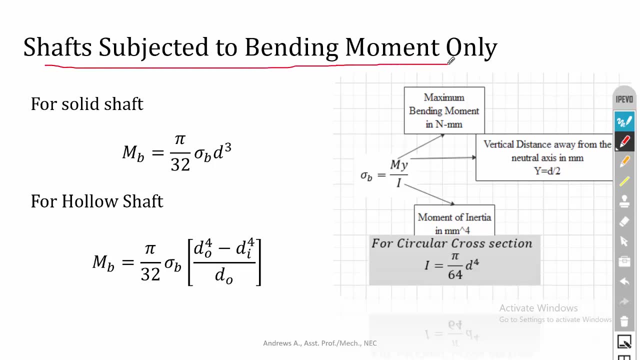 problems in the co1 in this case. so that is the shaft subjected to twisting moment only. so we have already solved few problems on this, so i am not going to solve any problems in the co2. and the next one is shaft subjected to bending moment only. so in the case of bending moment, we know that. 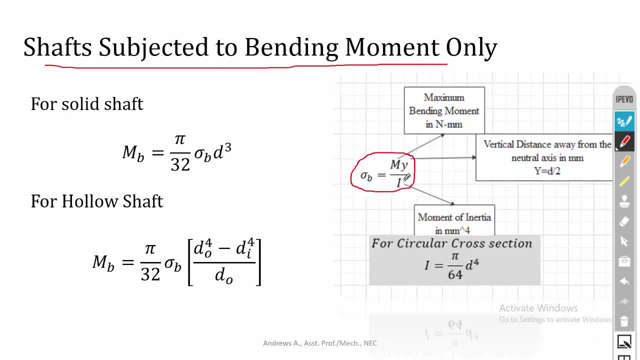 the bending stress. sigma b is equal to my divided by i, and here m is the maximum bending moment in Newton, mm, and y is the vertical distance from the neutral axis. in the case of circular cross section, we know that y is equal to d by 2 and i is the moment of inertia. 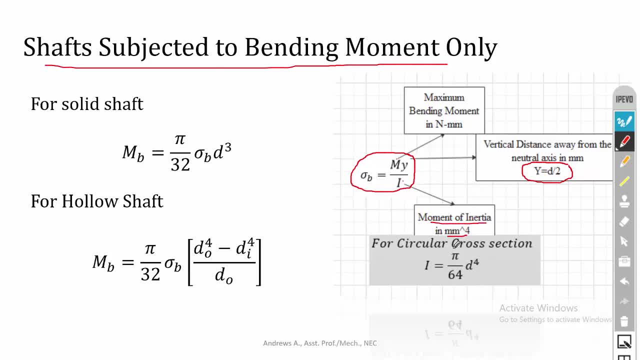 in mm power 4. and we know that for circular cross section, that is, solid circular cross section i, is equal to pi by 64 d power 4. so if we substitute everything then finally we will get. the mb is equal to pi by 32 sigma b, d, cube. 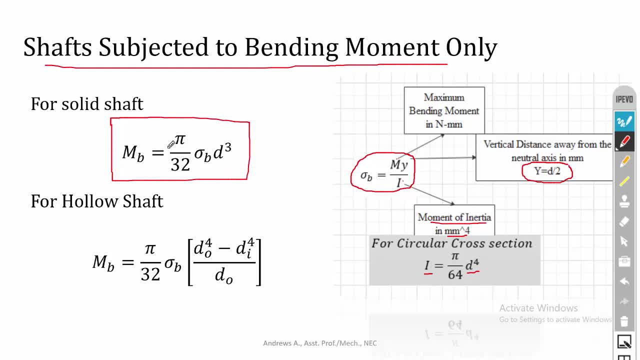 so or otherwise can write. sigma b is equal to 32 mb divided by pi d cube, so both are equal. so this is for a solid shaft and here mb is the maximum bending moment. sigma is: b is the allowable stress of the material and d is the diameter of the shaft. 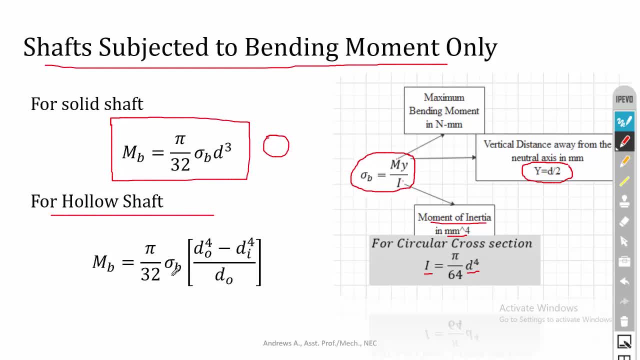 And in the case of hollow shaft, mb is equal to pi by 32 sigma b, outer diameter, power 4, minus inner diameter, power 4 divided by outer diameter. So this is for a hollow shaft.